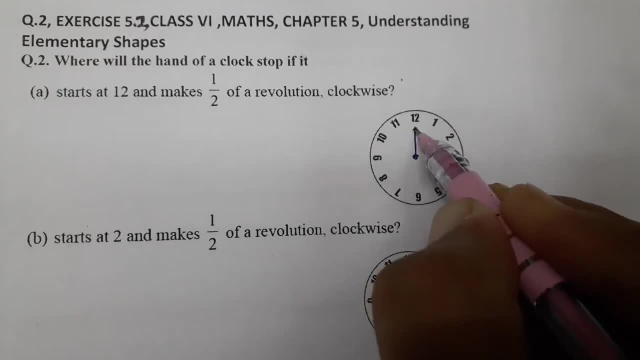 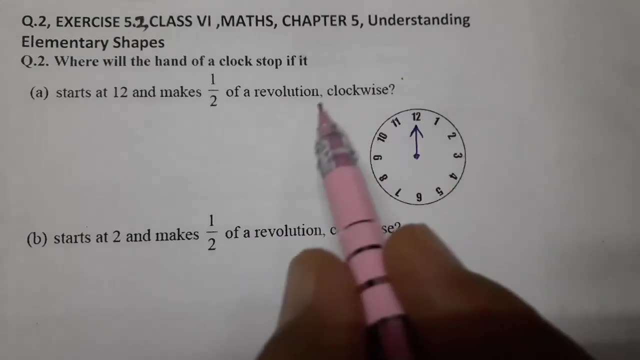 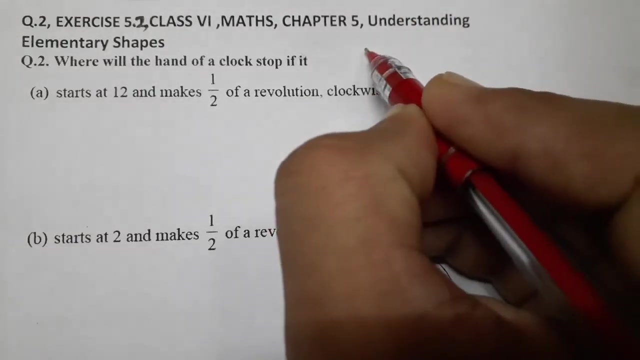 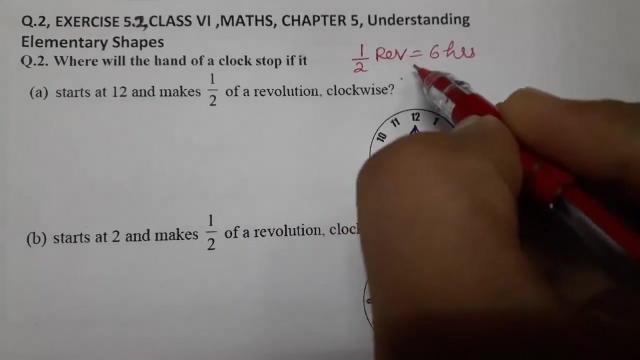 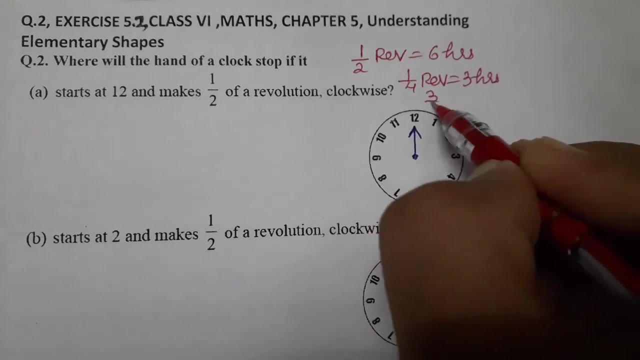 And makes half of a revolution clockwise. And we know, half revolution means 6 hours. So again, you must know all the things: Half revolution, 6 hours. One fourth revolution, 3 hours. Three, fourth revolution, 9 hours. 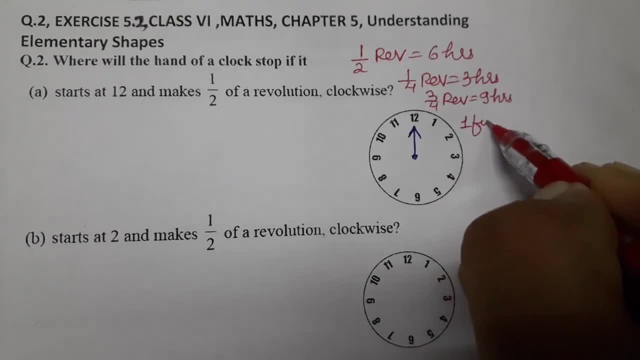 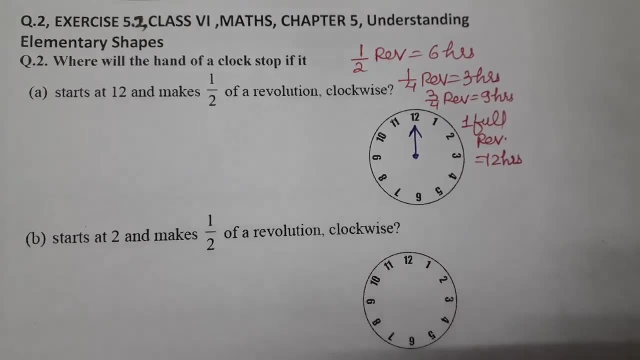 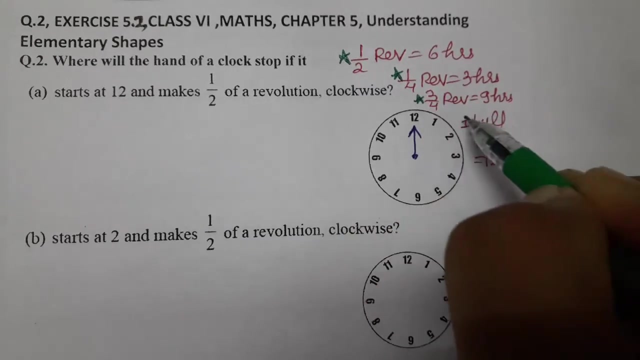 And last one, full revolution, 12 hours. So these are the key points. you must know. These all are 4 key points: 1,, 2,, 3 and 4.. So now let's start. Half of a revolution, clockwise. 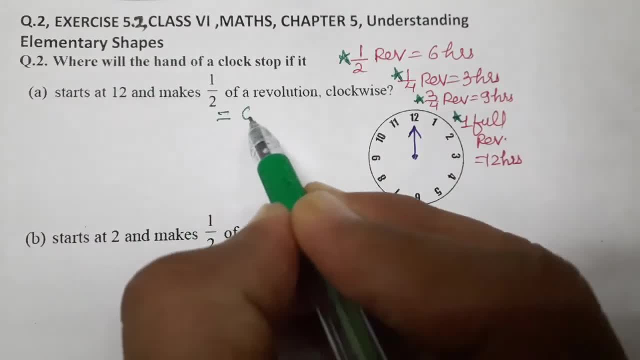 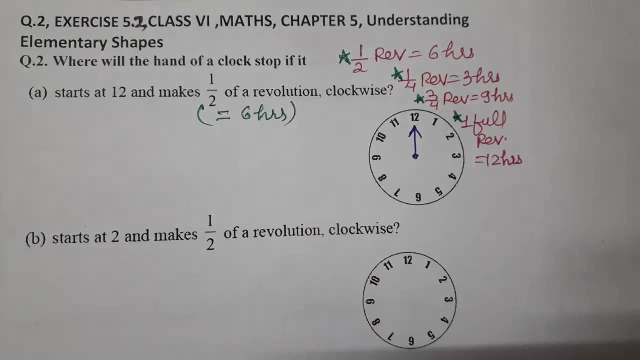 Half revolution means how many hours- 6 hours- We have to move towards 6 hours. So 6 hours. So let's move 6 hours: 1,, 2,, 3,, 4,, 5,, 6.. 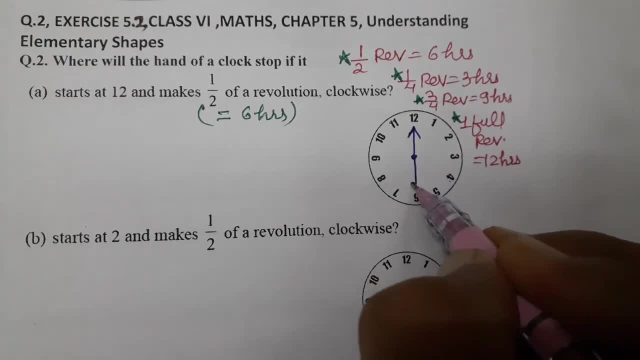 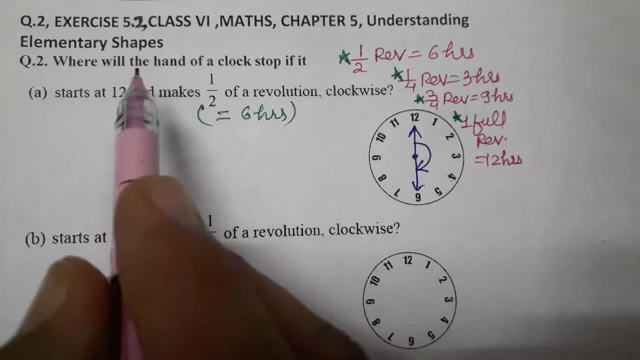 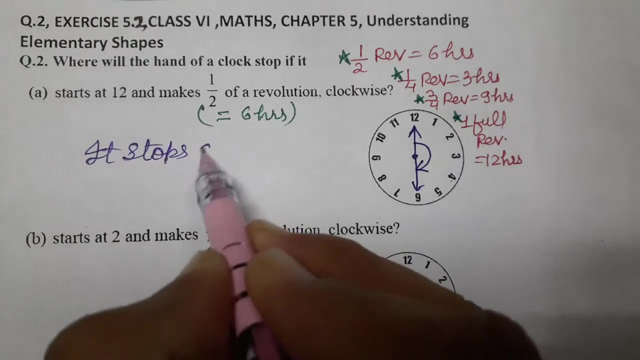 So we will reach at 6.. So this is 6 hours. So write where will the hand of a clock stop? So we will write it stops at 6 hours, 6 hours. starting at 6 hours, 6 hours. 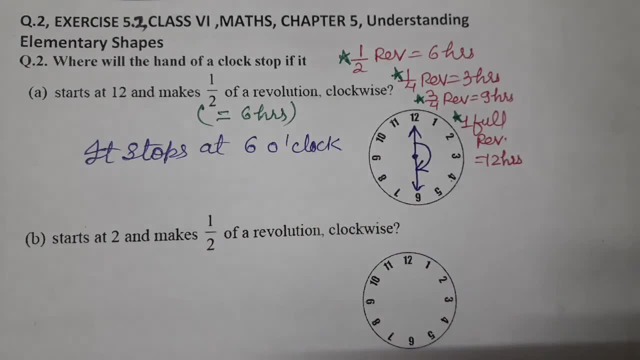 6 hours, Just in case, OK, We will write it from the line 1,, 2,, 3,, 4,, 5, 6.. 1,, 2,, 3,, 4,, 5, 6.. 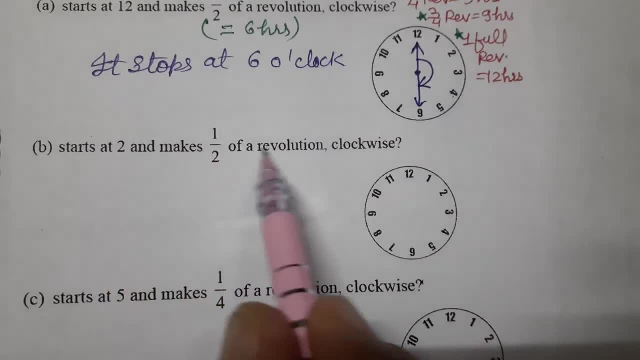 2,, 2,, 3,, 4,, 5, 6.. Stop at 1 point: 1,, 2,, 3,, 4,, 5, 6.. Stand at 5.. 2,, 2,, 3,, 4,, 5,, 6.. 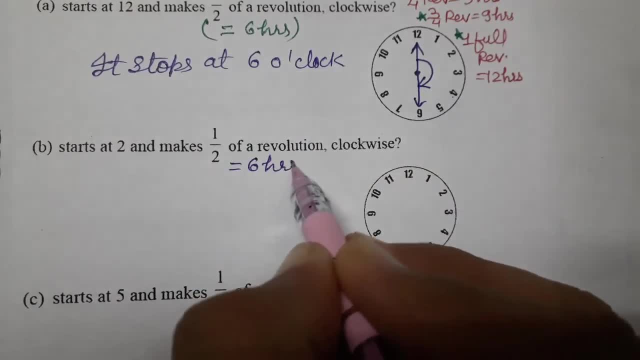 Now let's write the first one: 1,, 2,, three, 4, 6.. 1,, 2,, 3,, 4, 1.. Stop at 3.. 1,, 2,, 3,, 4,, 5,, 6.. 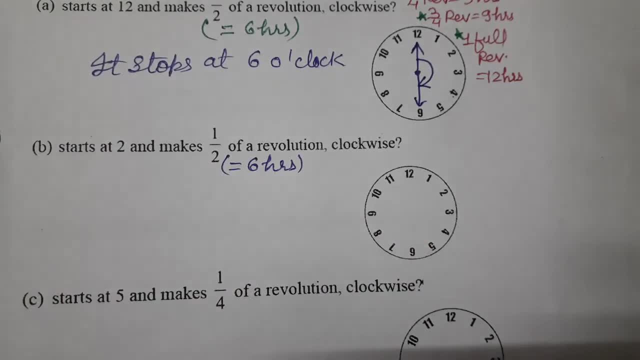 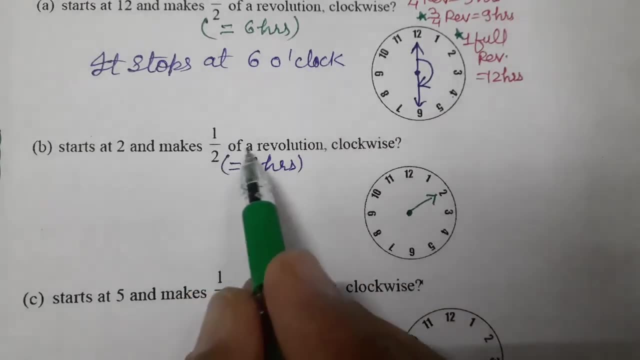 1,, 2,, 3,, 4,, 5, 6.. 1,, 2,, 3,, 4,, 5, 6.. where is to mark the center first, and this is two and makes half of a. 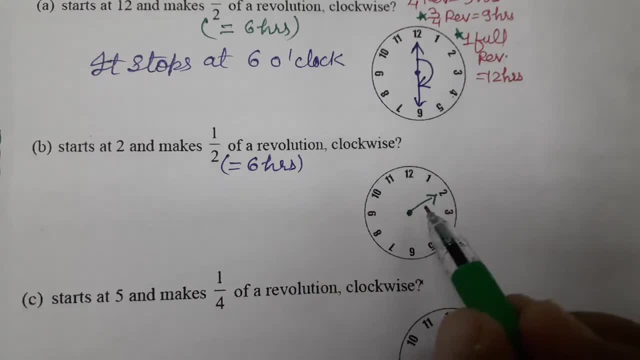 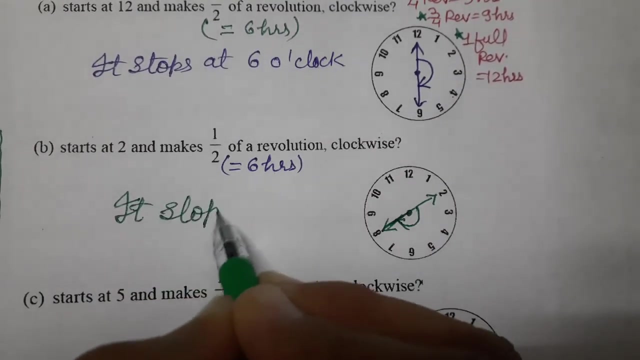 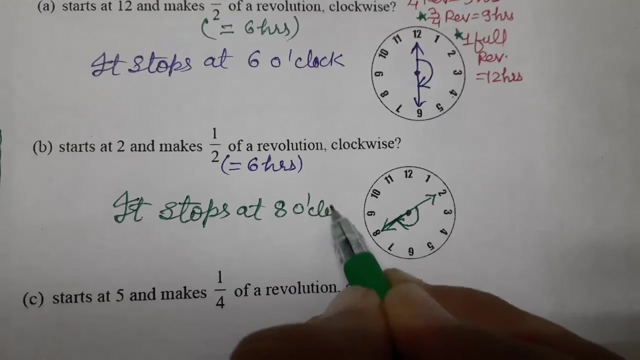 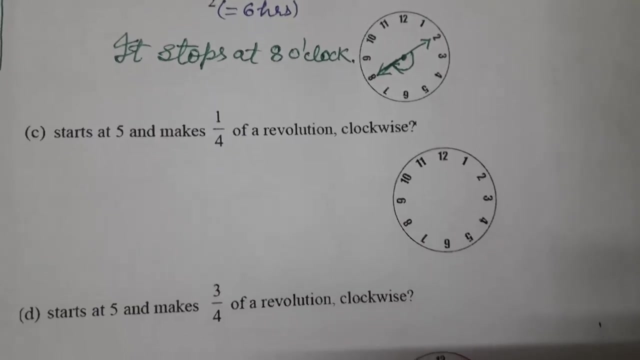 revolution. clockwise, clockwise, Jana. hey, six are Jana, one, two, three, four, five, six. so we reach at age. so we'll write. it stops at the clock. stop the hand of a clock. stops at 8 o'clock. next one, third one, c1. starts at 5 and makes 1, 4th of a. 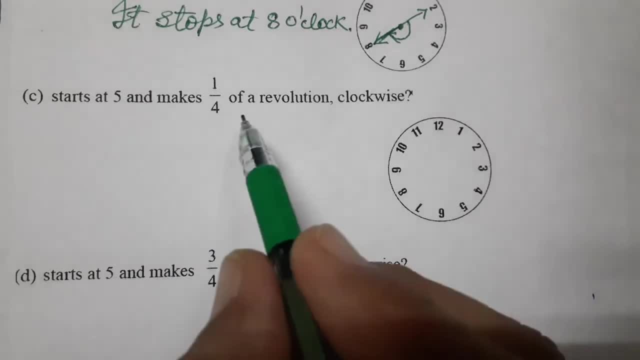 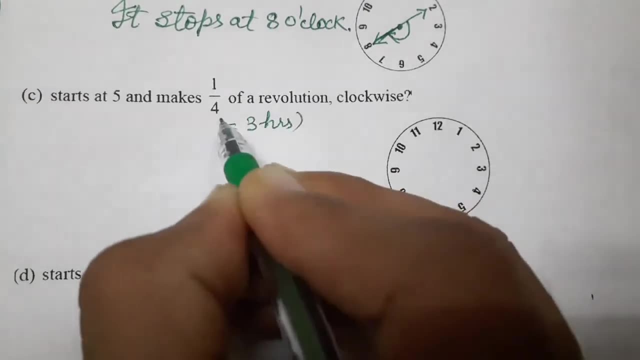 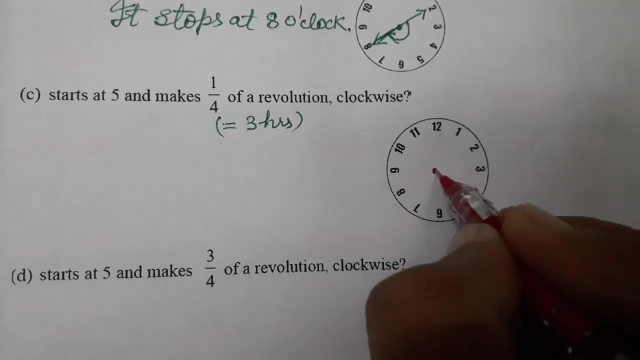 revolution clockwise. 1, 4th revolution. we know it is 3 hours. 1, 4th of a relation is 3 hours. now starts at 5. so where is 5c files here? 3 hours 1, 2, 3. so we'll write it. 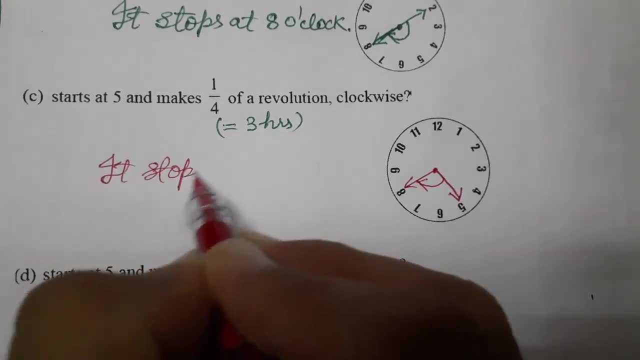 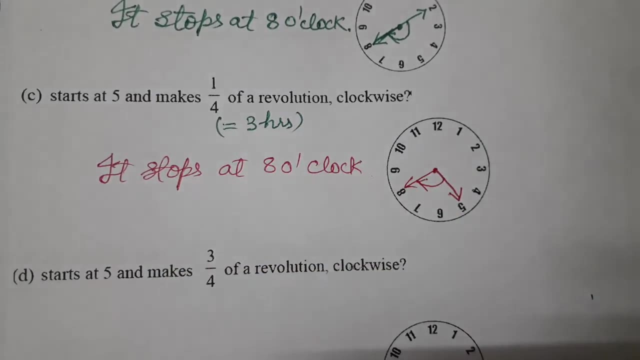 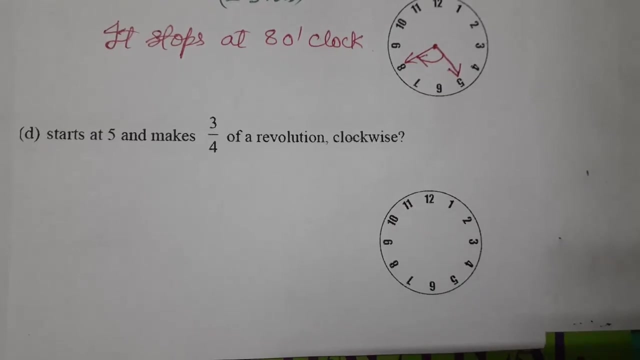 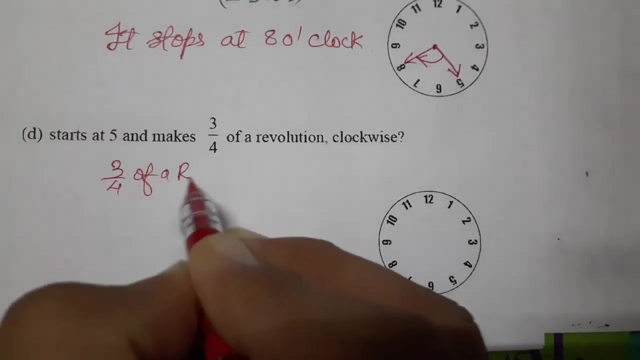 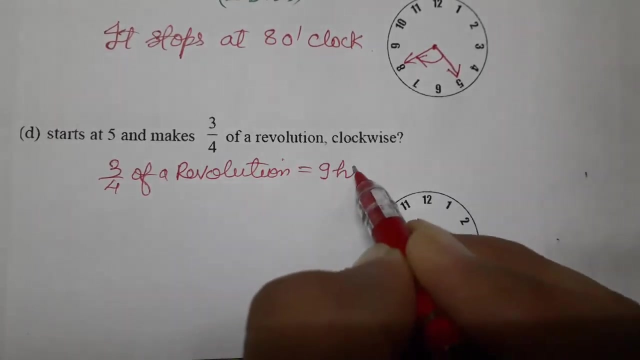 stopped. the hand of. a clock stops at 8 o'clock. now the D one it is starts at 5 and makes three, fourth of a revolution clockwise. and we know three, 4th of revolution means three, fourth of a revolution equals to nine hours. so let's start from five only. 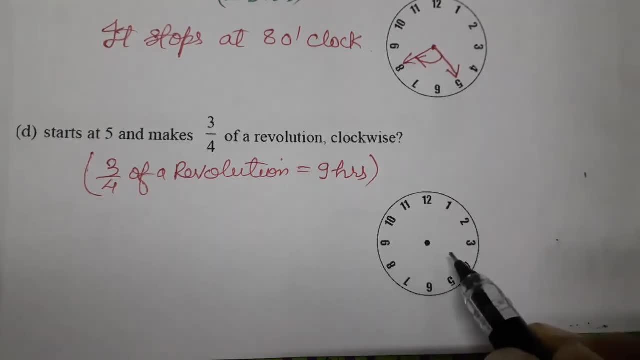 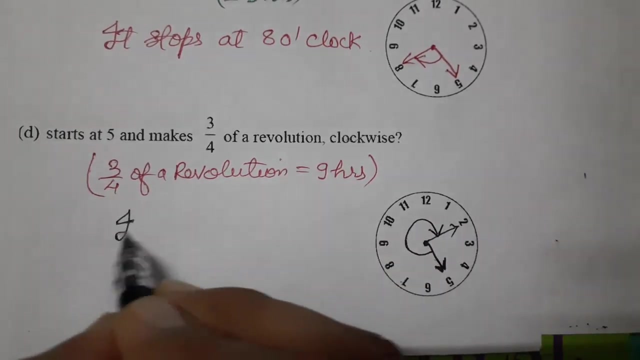 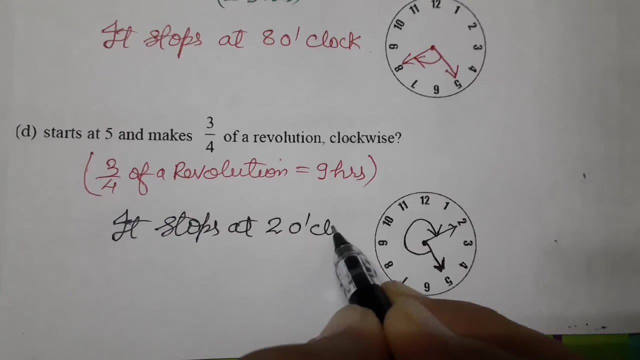 you. it is 5 now, 9 hours. 1, 2, 3, 4, 5, 6, 7, 8, 9, so we reach at 2. so we have to move clockwise every time. so it stops at the hand of a clock, stops at 2 o'clock. so I 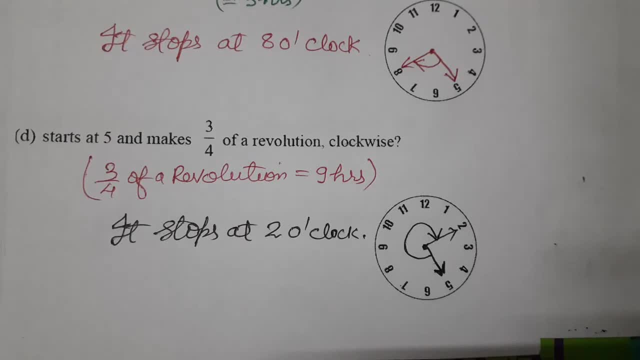 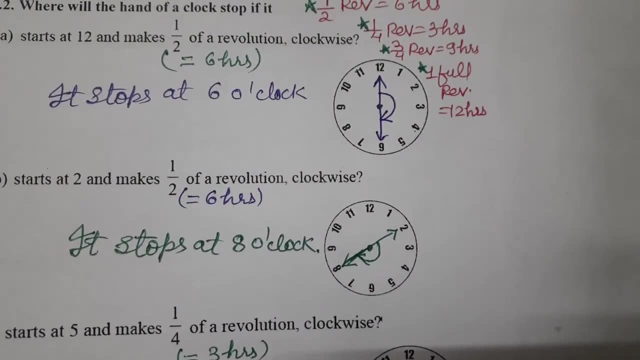 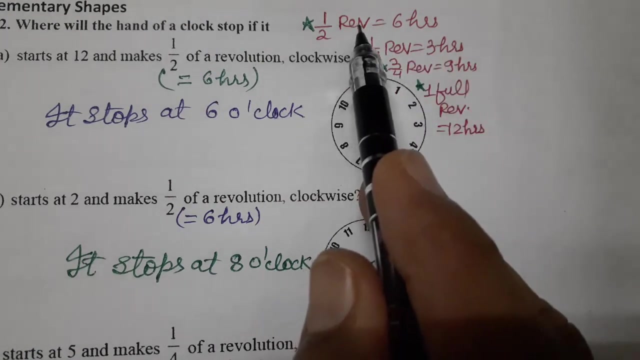 hope you understood how we have to move. we have to only remember the key points and the key points that we have written also, and you must know the key points before doing the question. 1: 4th revolution: 3 hours, 1 right angle, half revolution, 6 hours: 2 right angles or 1 straight angle.